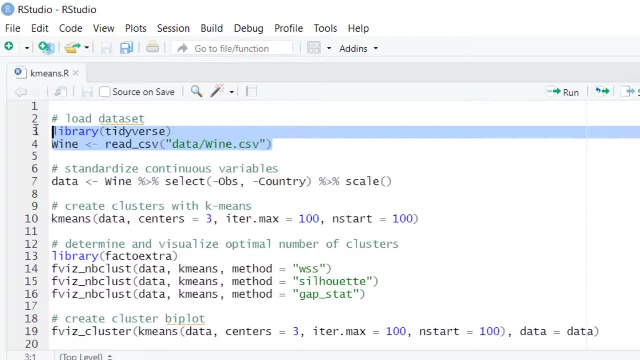 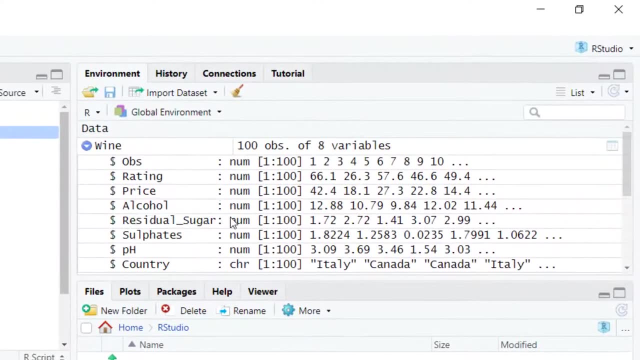 with the k-means function. I'm going to do an example here and I'm going to use the wine dataset. In this dataset we have information about several wine brands. We have data about our rating products: alcohol, residual sugar, sulfates. 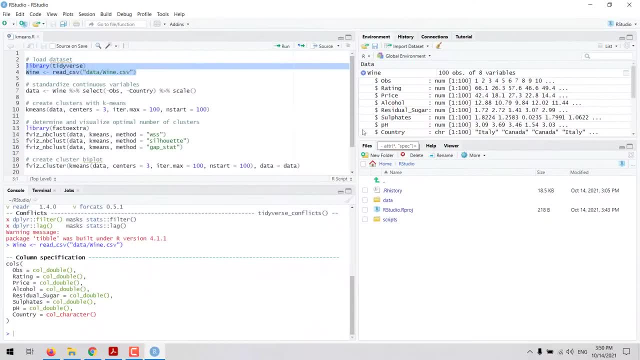 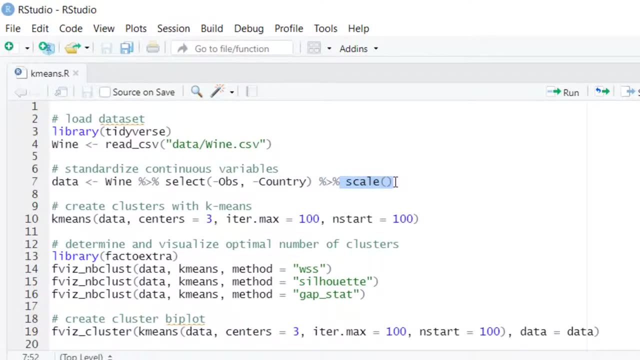 and pH, And we have some categorical variables that I'm going to remove here. I'm going to remove them And then I'm going to standardise the continuous variables. This step is important to avoid that variables with a larger range of values have more influence on the results than variables with a shorter range of values. 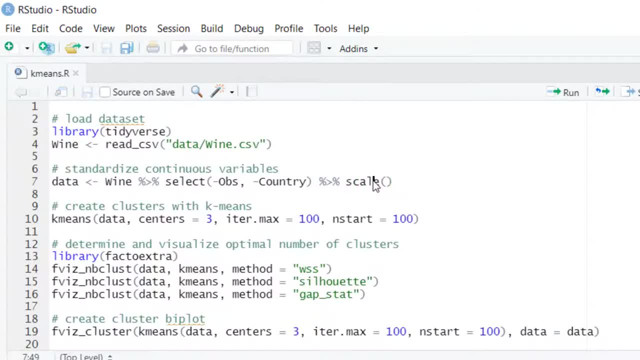 So what we do here is that we center the data around the mean and then we divide by the standard deviations of each variable, so then each variable will have standard deviations as units. Okay, let's run this code and then let's work with the k-means function. 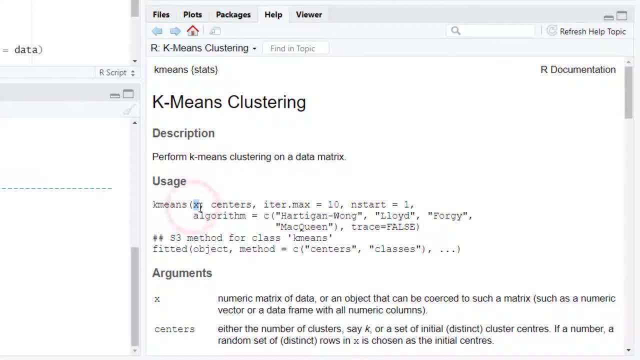 In this function we are going to need to enter first the dataset, then we enter the number of centers or clusters that we want to create. So this is defined by the user. We can ask for 2,, 3,, 10, or more clusters. 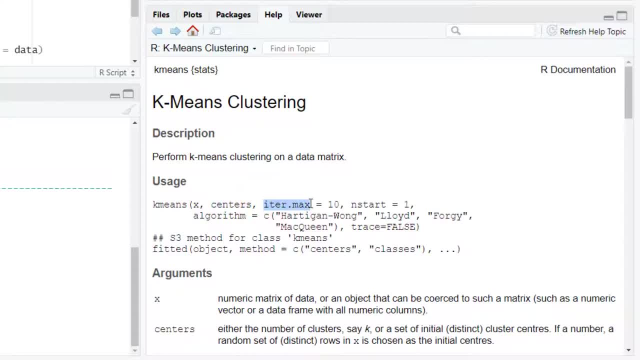 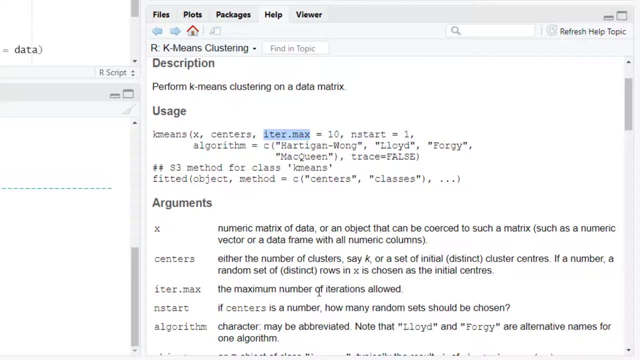 Other arguments here, for example, are the maximum number of iterations. We can set this, for example, to 100.. Or we could use this nstart argument to define the number of random sets that should be created. So r will create a given number of random sets and at the end will keep the set that produces the best results. 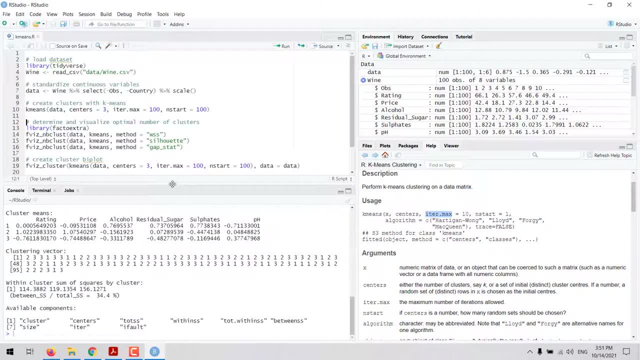 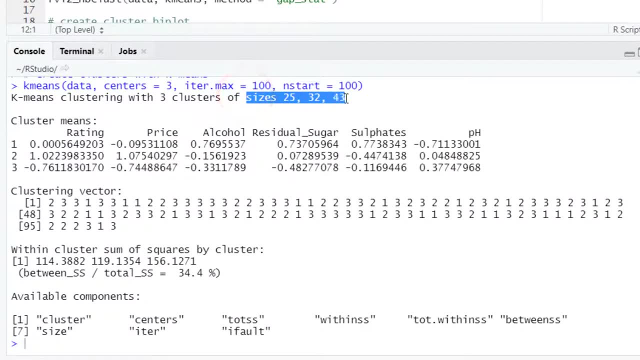 Okay, So okay, let's run this code and let's see the output here. So we are running k-means clustering with 3 clusters. Here we see the number of observations in each of the clusters. Then we see this table with the cluster centroids. 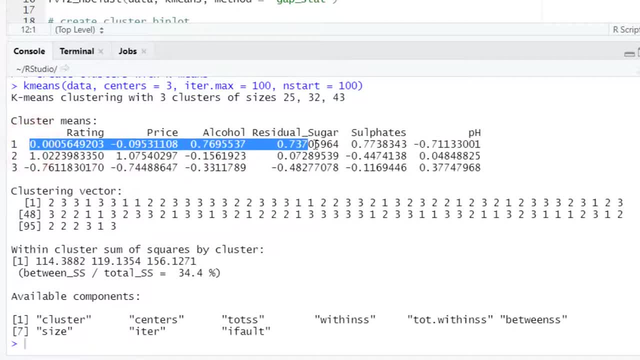 So each of the rows here in this table is one cluster and this will be the corresponding centroid. So this will be the average value for each of the variables in the observations in that cluster. So For example, we can see that if we examine, let's say, the rating variable, then the average would be 0 for this first cluster. 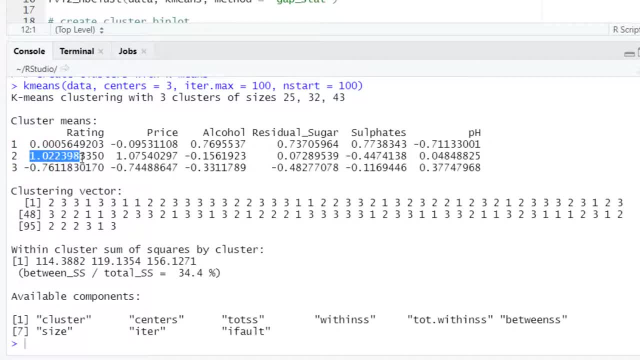 Then the average for rating variable in the second cluster would be close to 1,, while the average for the same variable in cluster 3 would be negative and around 0.8.. Then we can take a look at this clustering vector. This is a vector that shows to which cluster each observation in the data set will be assigned. 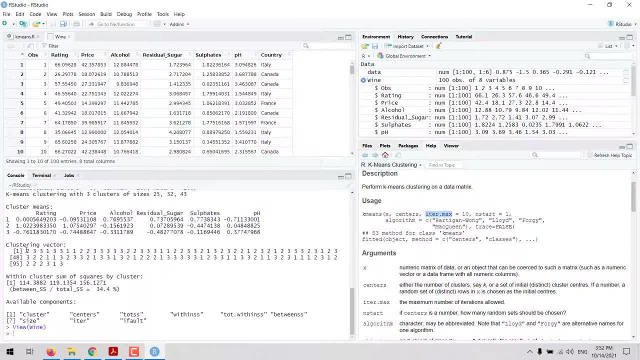 So let's say that here we have our DeWine data set and then this means that the first observation in the data set will be assigned to cluster 2.. So this first observation will be assigned to cluster 2, and then observations 2 and 3. 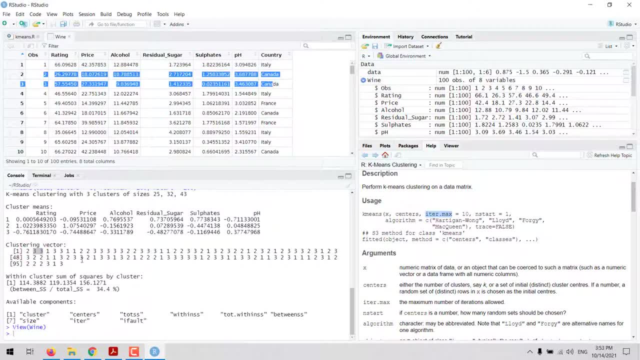 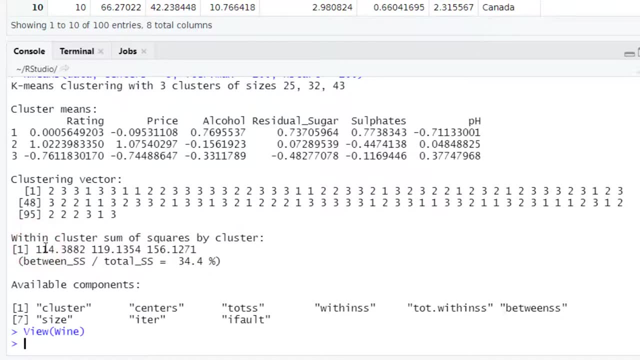 will be assigned to cluster 3, and so on. We can also see here the within-cluster sum of squares. This can be used, for example, for defining the best value for k, so we will try to minimize the total within sum of squares. 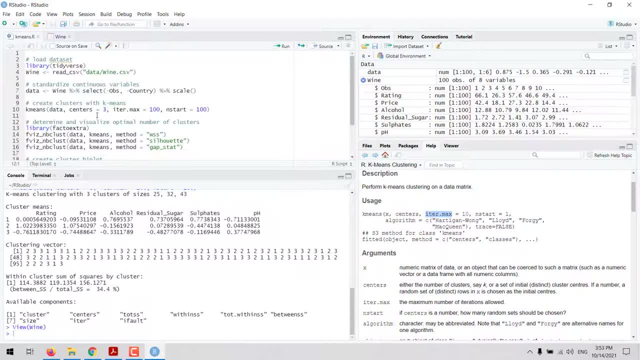 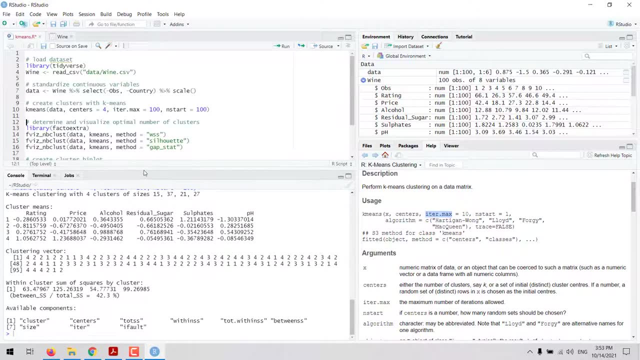 We can also see here the within-cluster sum of squares. In our script we could try, for example, a different value for k over the number of clusters. let's say this, and then we would get a slightly different result for clusters and then the clustering vector and then the within-cluster sum of squares. 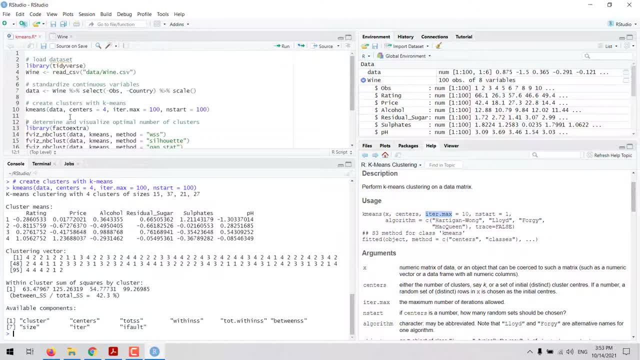 So we could try different values for k. we could use a for loop and then, let's say, evaluate values for k between 2 and 10 or more. We could do that manually or we could use some patterns. We could do that manually or we could use some patterns. 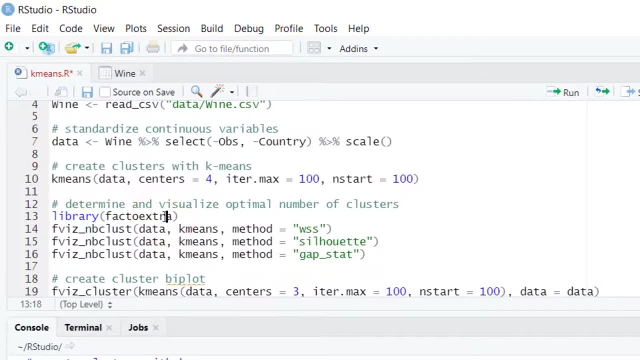 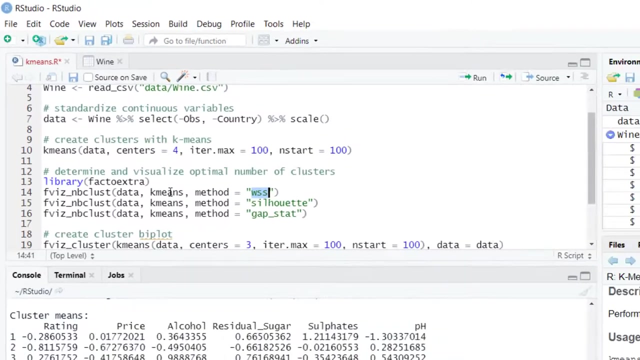 packages that provide that functionality, for example this factor extra package. this can help us to evaluate the. this case means clustering algorithm for different values of k. there are different methods for selecting the best value for k. here, for example, we have these methods: the within sum of squares, the average silhouette width or the gap statistic. so if we try with the 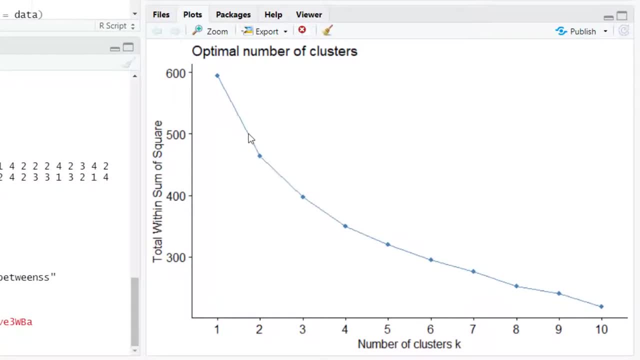 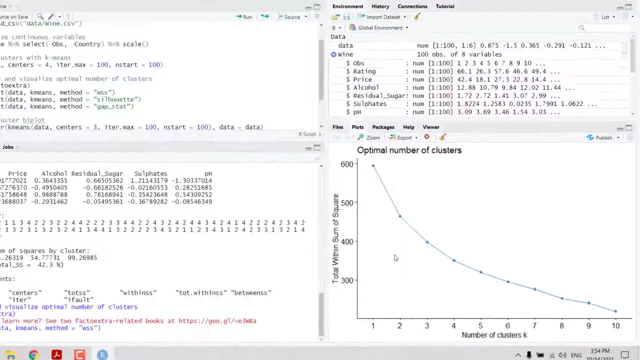 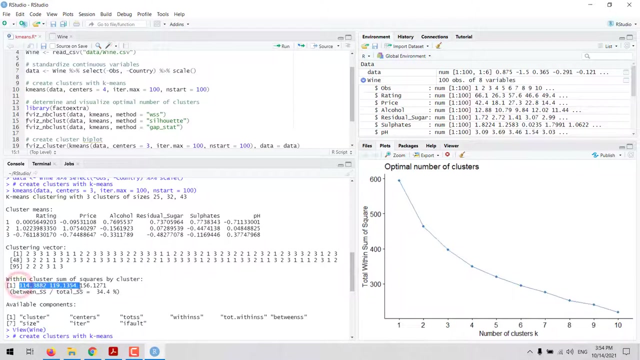 first method, wss, we get this chart. so we got the number of clusters in the x-axis and the total within some squares in the y-axis. so, for example, when we run this algorithm for k equal to three, then we got this within clusters of squares which the total value would be around 400, which is 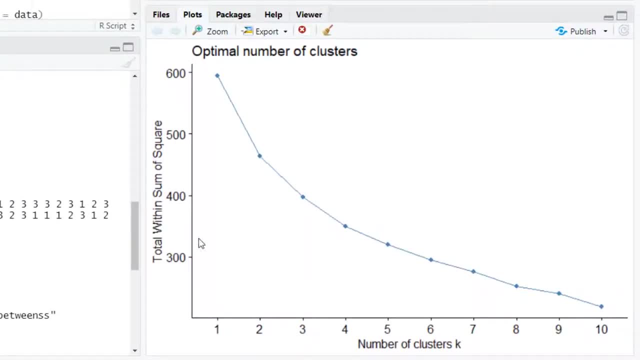 the value that we see here for three. to define the optimal number of clusters we would use the elbow rule or knee rule, so we will try to find after which number of clusters the total within some squares does not decrease much, and then at that point we would select the optimal number of. 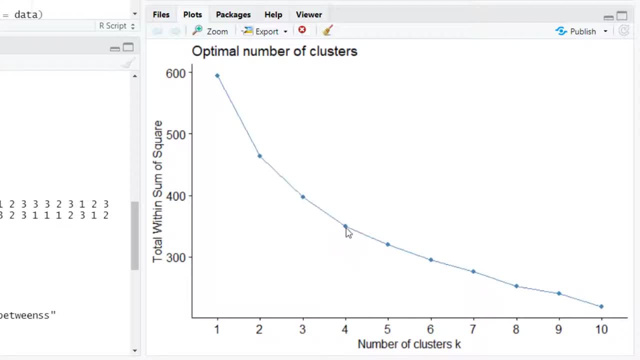 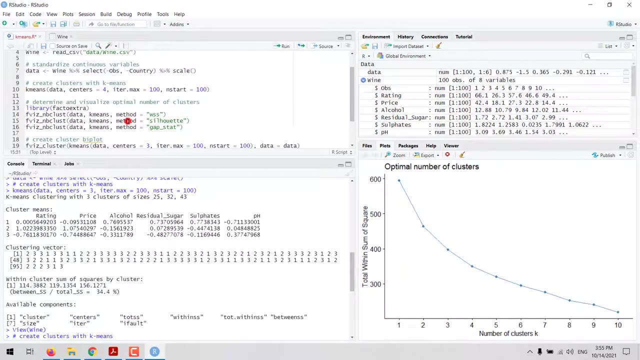 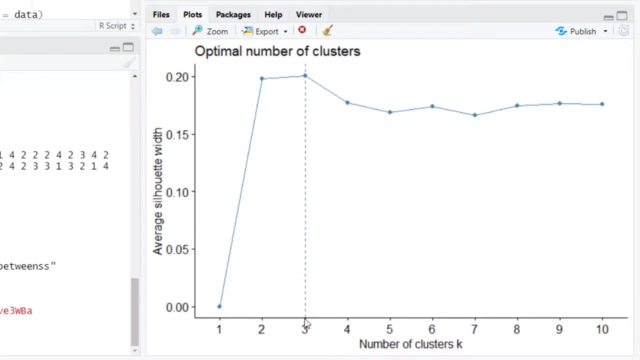 clusters. let's say here after three or four clusters, then the total within some squares does not decrease as much as before. so that would be the first method, or we could try it with the average silhouette width method. here we see that the optimal number of clusters don't exceed very much. but more or less to true is 2 and ok. now we sorrow that. 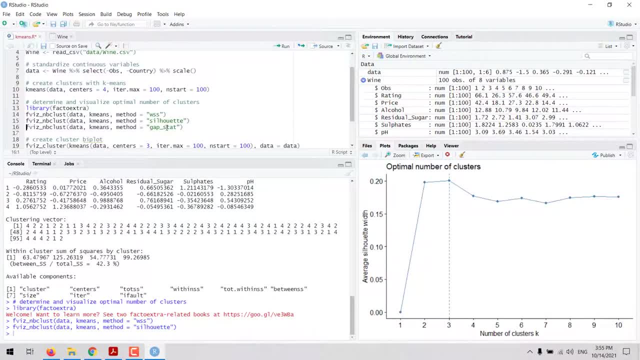 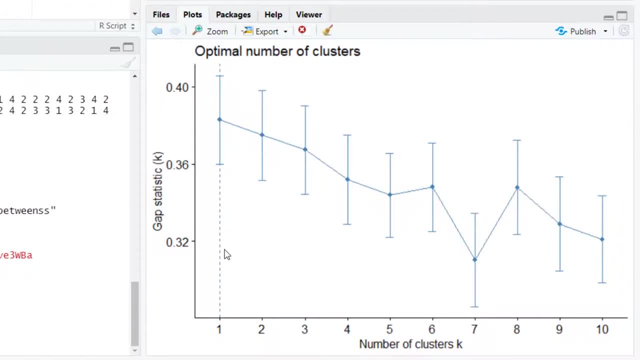 f prime into the nextidée. with f prime, transpose is less than one. now if we see the hell problem here in the chart, let's say there is some value in thericht. and if we see that here we see that f prime another variable for this method. and when i change the number of clusters, 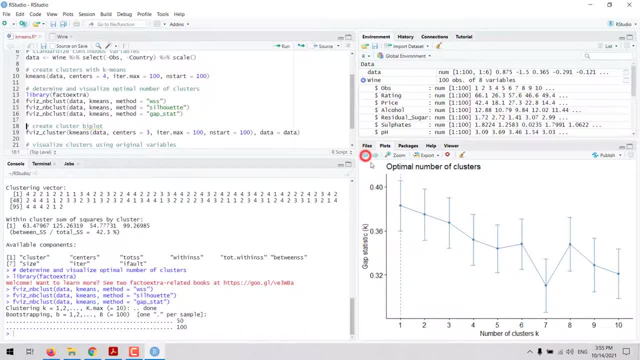 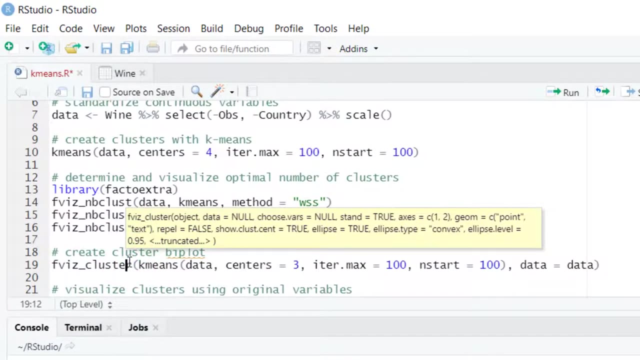 think it makes more sense for your data. let's say here we can work with the silhouette method and we would define three as the best value for k. then we could analyze a cluster by plot. so we can create a cluster by plot in r with the fb underscore cluster function. we will enter 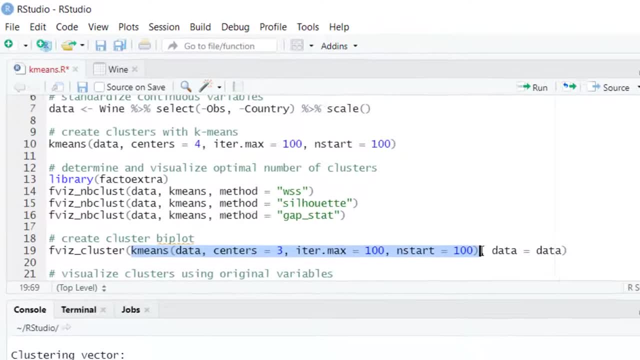 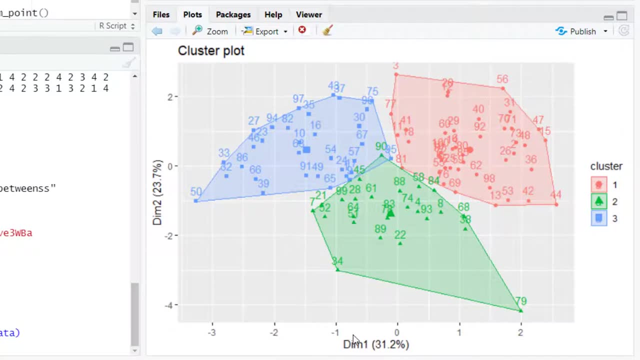 the k means function with the desired number of k and then if we run this we get the by plot. so here you can note in the axis that we have the first principal component in the x-axis and the second principal component in the y-axis. the number in parentheses would be the amount of 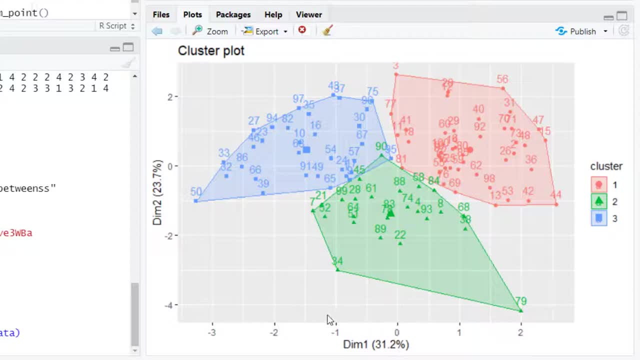 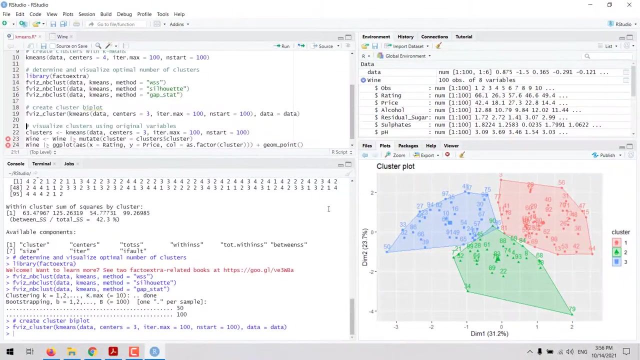 variability that is explained by each of the components. so here we can see how these clusters are well separated. so we have first cluster in color red here, then we have the second cluster in green and the third cluster in black in blue. if we change the number of clusters to four, let's see how this cluster plot looks like. 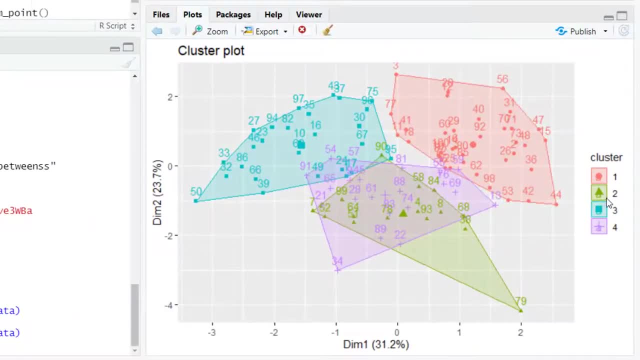 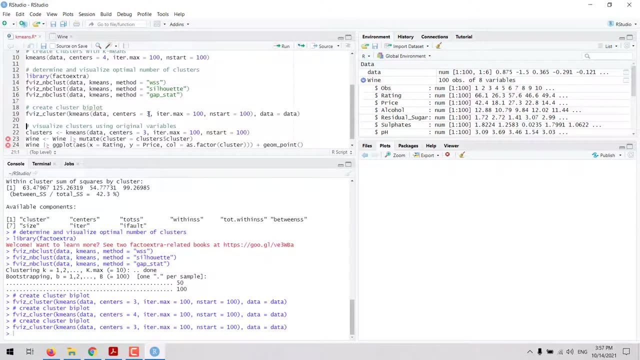 for example, here we would see that clusters 2 and cluster 4 overlap. so let's say that we would prefer to work with three clusters. okay, after that, instead of using the principal components as variable for the access, we could create a similar plot using the original variables.